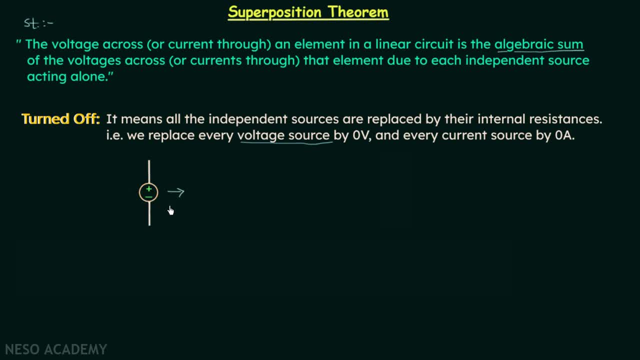 we have this voltage source and if we want to turn off this voltage source, then we will simply short circuit this voltage source. Here we have short circuited this voltage source and if we have the current source and we want to turn it off, then we will open circuit this current source. Here we have. 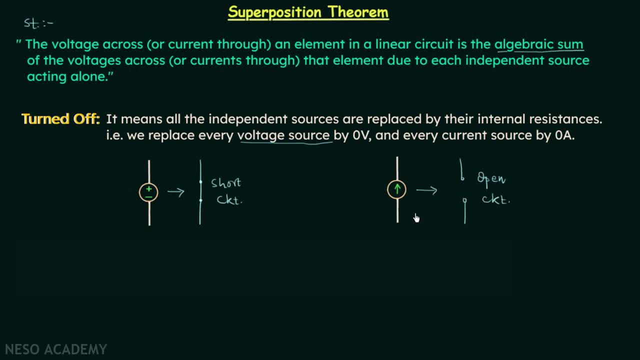 open circuited this current source. So this is what do we mean by turning off the independent sources. Now, before we move on to the example, to understand the superposition theorem in a better way, we will first note down 2 important points. According to the first point, we do not turn off. 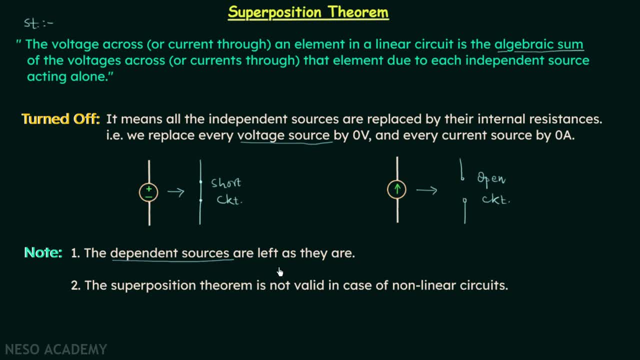 the dependent sources. The dependent sources are left as they are. This is important point to remember. in second point, we should note down that the superposition theorem is not valid in case of non-linear circuits. so this is all for the introduction. now we will move on to the 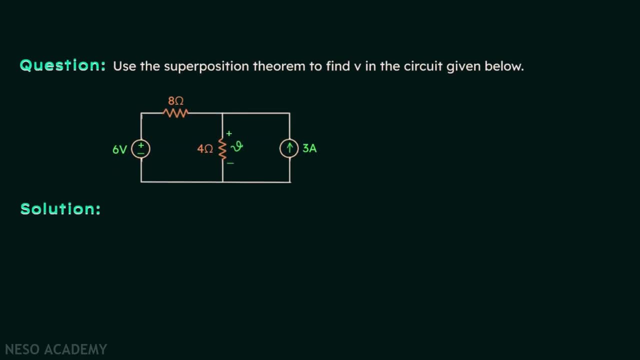 implementation and i have taken one question to understand how we can use superposition to find the voltage across an element. so here is our network and we need to find this voltage v by using the superposition theorem. i will give you few seconds to analyze the given network. 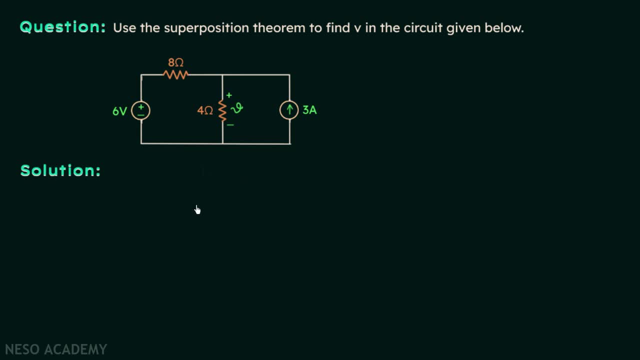 i hope you are done now we will move on to the solution. when you observe the given network, you will find we have one and two sources and we have two resistors, out of which we need to find the voltage across four ohm resistor and for this purpose, 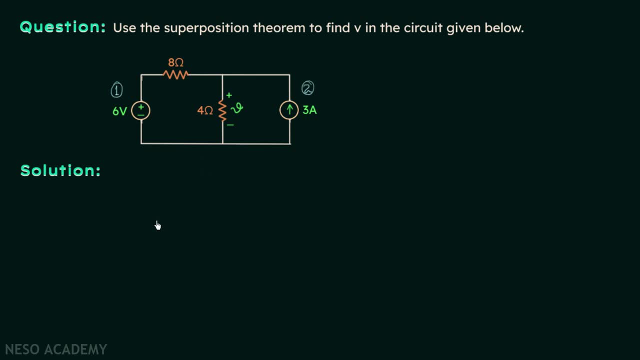 we are going to use the superposition theorem. i will give you a few seconds to analyze the given. we will use superposition theorem and, according to the superposition theorem, the voltage across an element is the algebraic sum of the voltages due to each independent source acting alone. we 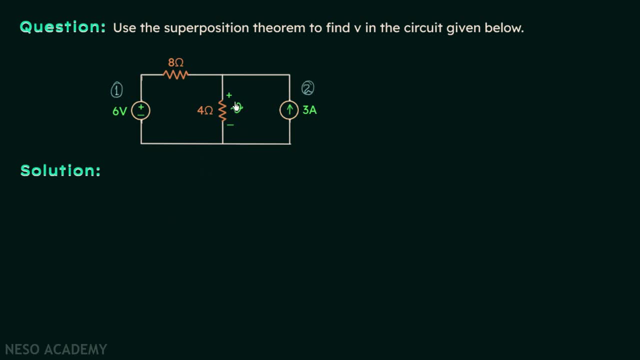 have two independent sources and we need to find out voltage across this resistor due to each source, one by one, and then, finally, we will add the obtained voltages to have the net voltage v. this will be more clear once we start solving the question. so what i will do first is i will consider the voltage across four ohm resistor due to this source. 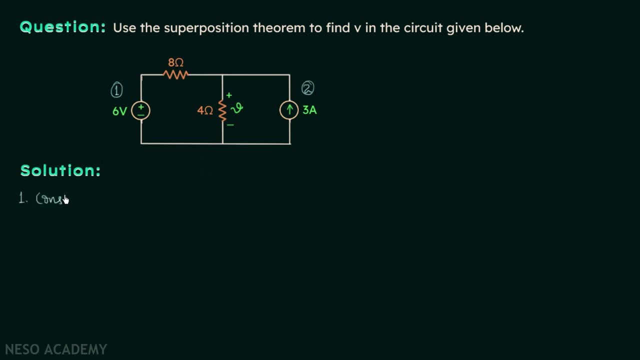 so first i will consider the six volt source, and this means we need to turn off this three ampere source. that means we will open circuit this source. so let us copy the given network and after copying it we will do some modifications, and the modification is we will open circuit this. 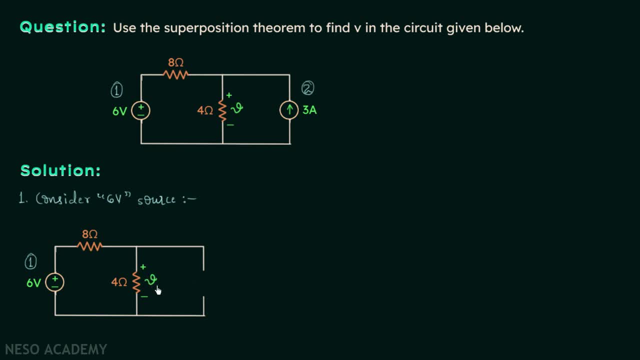 source and we will write v as v sub 1, because this is not the voltage v. we have turned off this source and therefore the voltage obtained here is only due to this source. now it is very easy to find out v1. if we can find out the current through this resistor we can have. 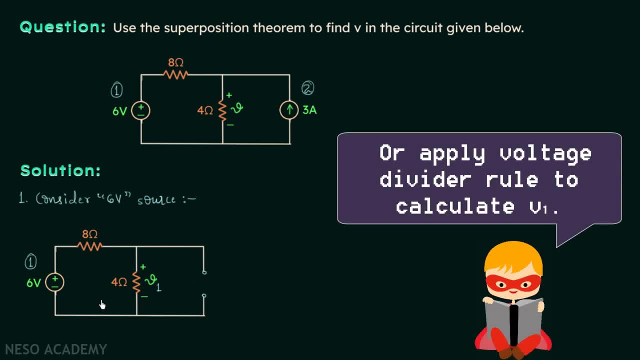 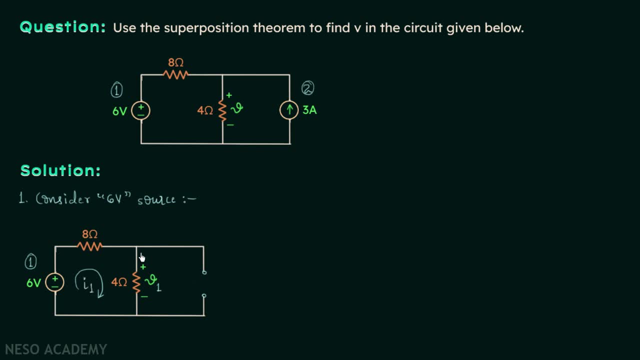 v1 and to find out the current. in this loop we will first assume the current to be i1 and then we will apply kvl. after applying the kvl, we will have plus 6 volts, minus i1, multiplied to 8, minus i1, multiplied to 4, equal to 0. so we will have i1 equal to 6 divided by 8 plus 4, or we can say that: 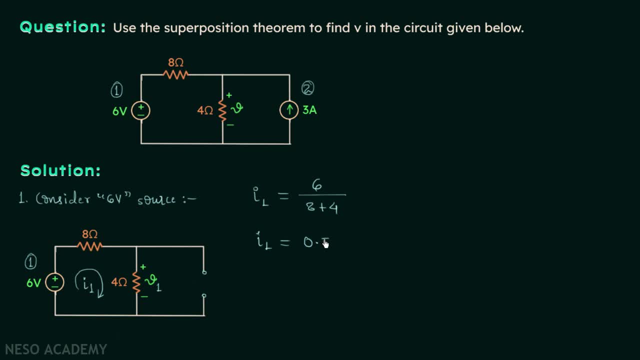 current i1 is equal to 0.5 amperes. now v1 it is equal to i1 multiplied to 4. we know i1 it is 0.5. therefore, v1 is equal to 0.5 multiplied to 4, that is 2 volts. so in this way we have obtained: 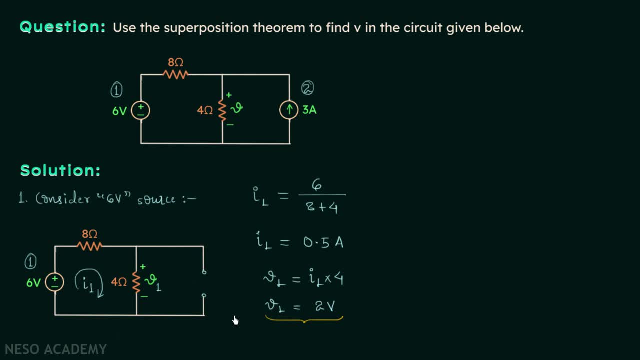 v1, which is voltage across 4 ohm resistor due to 6 volt source alone. now we will find out the voltage across 4 ohm resistor due to this source. so this time we will consider the 3 amperes source and this means we need to turn off the 6 volt source. so again, we will do the 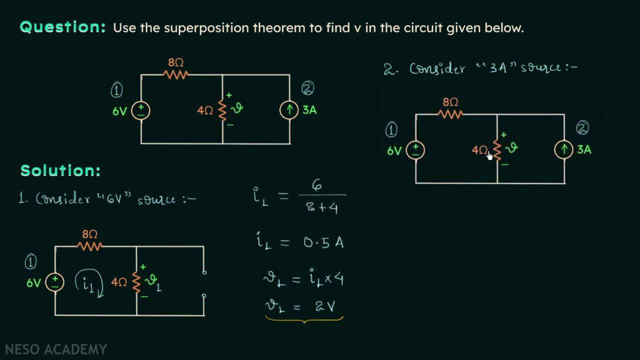 modification in our network and this time we are going to short circuit the 6 volt source. so i will remove this source and then we will have a short circuit, short circuit plus. i will change the name of v. we will call it v sub 2. now again, we will focus on 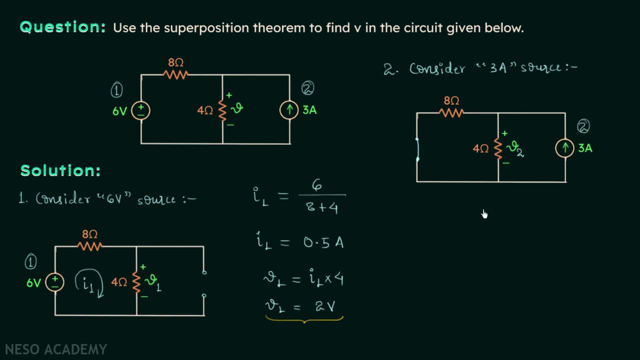 the calculation of voltage across this resistor. but this time we will find it out due to this source here. when this source is turned off, and to find out the voltage v2, we will first find out the current in this branch. let's say the current is i2. 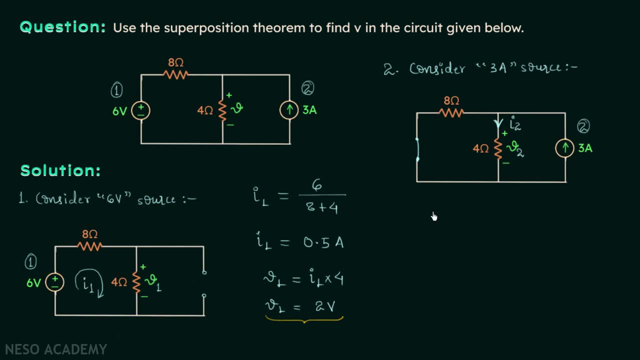 we can have V2.. To find out I2, we will use the current divider rule. According to the current divider rule, we will have I2 equal to the total current entering multiplied to the other resistance, which is 8 ohms divided by the sum of two. 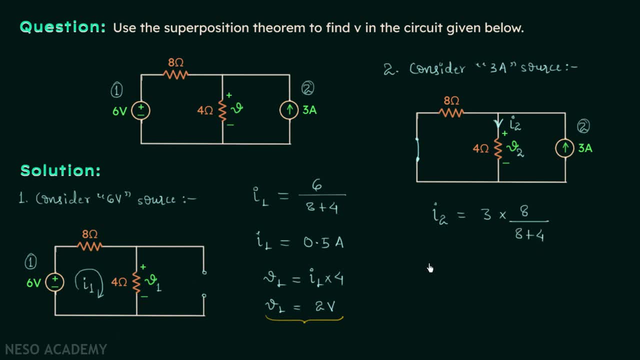 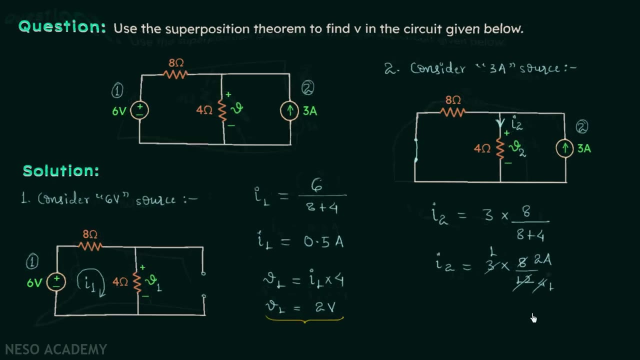 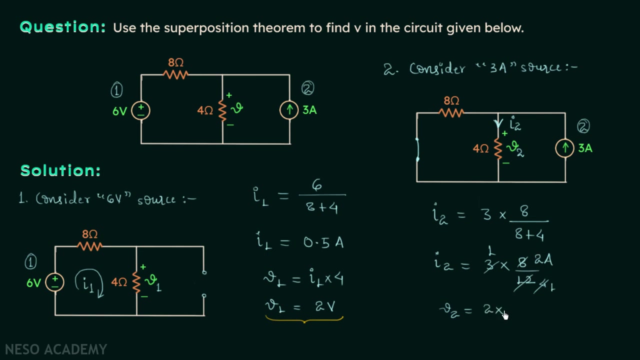 resistances 8 plus 4.. So we have I2 equal to 3 multiplied to 8 divided by 12. so in this way we have obtained I2 equal to 2 amperes. Now we can find out V2.. V2 is equal to I2, which is 2 multiplied to 4 ohms. So finally we are. 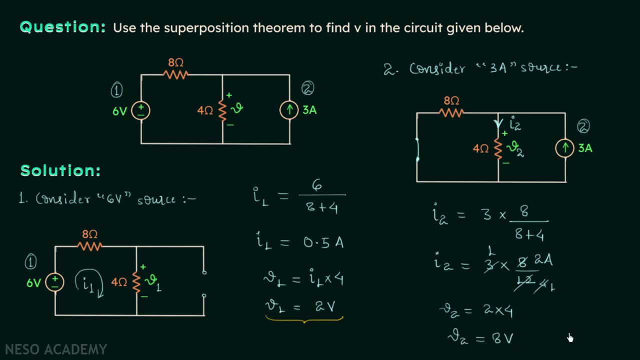 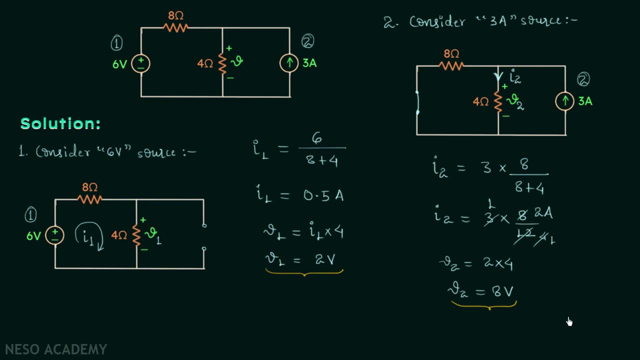 getting V2 equal to 8 volts. So 8 volts is the voltage across 4 ohm resistor because of this 3 ampere source. Now the net voltage across this resistor, which is V, is equal to V1 plus V2. and this is from superposition theorem. We know V1, we know V2.. We will have V equal to 2 plus 8.